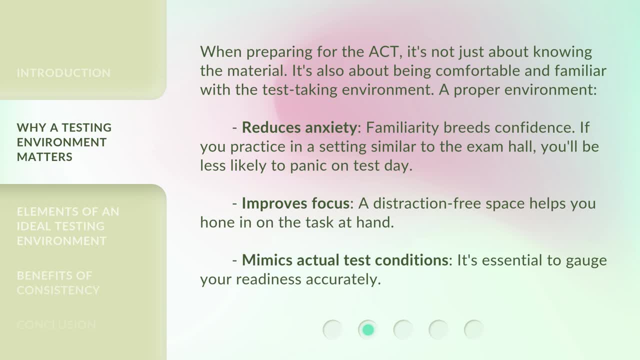 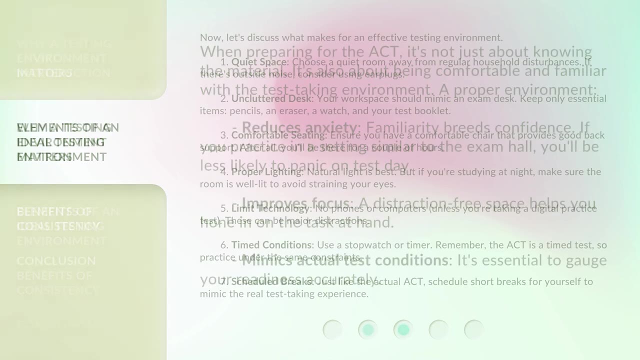 you'll be less likely to panic on test day. Improves focus: A distraction-free space helps you hone in on the task at hand. Mimics actual test conditions. It's essential to gauge your readiness accurately. Now let's discuss what makes for an. 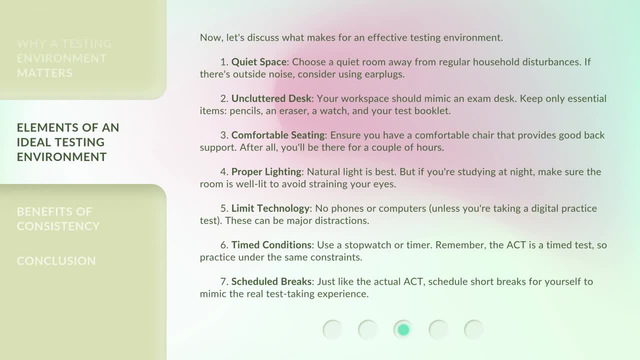 effective testing environment. 1. Quiet space. Choose a quiet room away from regular household disturbances. If there's outside noise, consider using earplugs. 2. Uncluttered desk. Your workspace should mimic an exam desk. Keep only essential items: Pencils, an eraser, a watch. 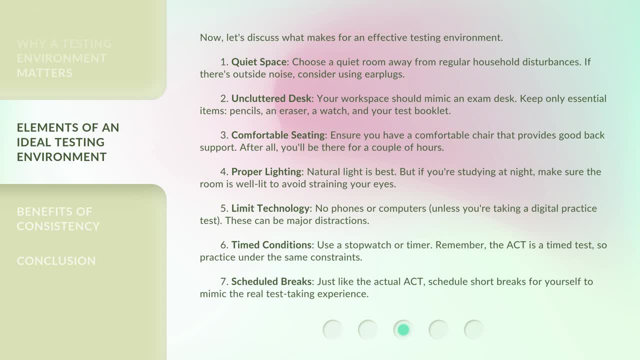 and your test booklet. 3. Comfortable seating: Ensure you have a comfortable chair that provides good back support. After all, you'll be there for a couple of hours. 4. Proper lighting. Natural light is best, But if you're studying at night, make sure the room is well lit to avoid straining. 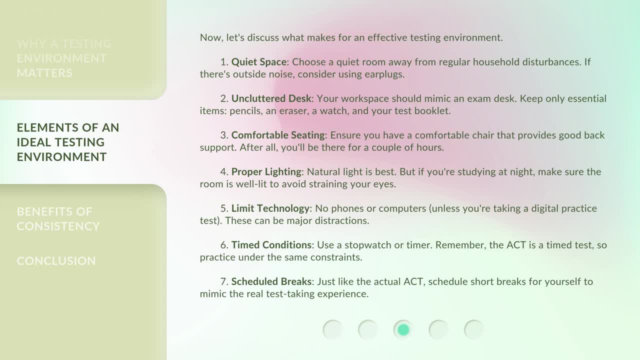 your eyes. 5. Limit technology: No phones or computers unless you're taking a digital practice test. These can be major distractions. 6. Timed conditions: Use a stopwatch or timer. Remember the ACT is a timed test, so practice under the same constraints. 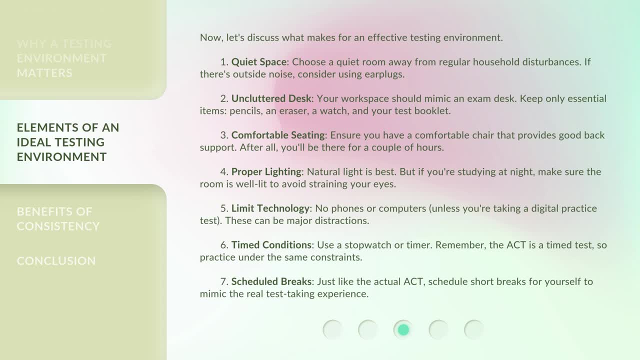 7. Scheduled breaks Just like the actual ACT schedule. short breaks for yourself that you just took in the morning or morning to mimic the real test-taking experience. 6. Spontaneous practice: Don't do sleep test to help with the test. 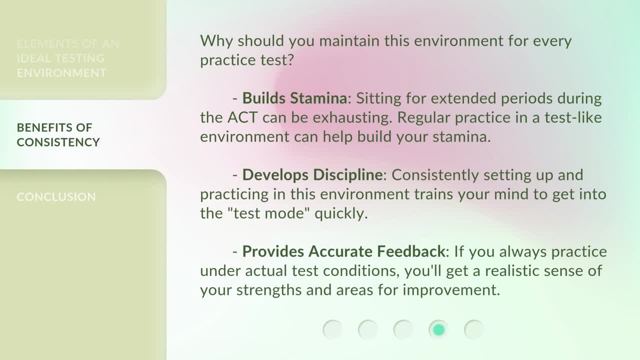 Why should you maintain this environment for every practice test? Build stamina. Sitting for extended periods during the ACT can be exhausting. Regular practice in a test-like environment can help build your stamina. 7. Develops discipline. Consistently setting up and practicing in this environment trains your mind to get into the test mode quickly.